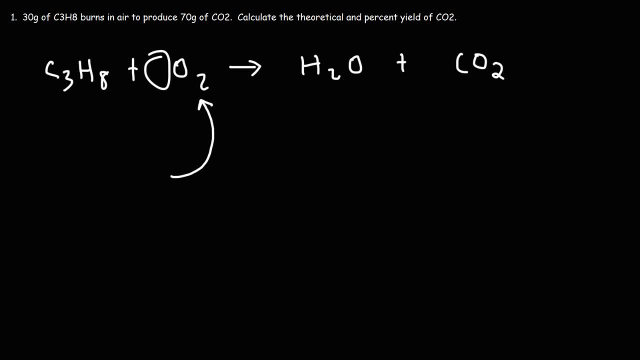 put a number in front of O2, you're only changing the number of oxygen atoms on the left side. So that's why you want to save this for last is because it's the pure element in this chemical reaction. So let's begin by balancing the carbon atoms first. We have three carbon atoms on the left side. 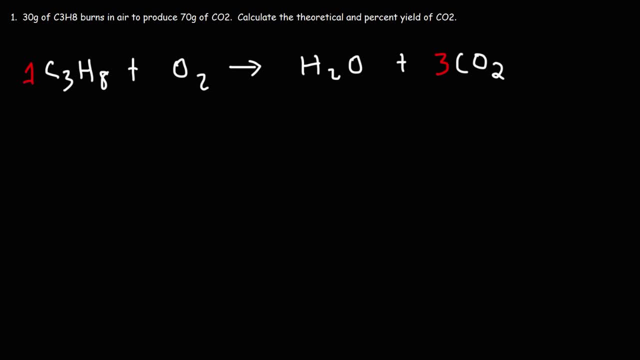 We only have one on the right side, So to make them equal we need to put a three in front of CO2.. Next let's move on to the hydrogen atoms. We have eight hydrogen atoms on the left side, only two on the. 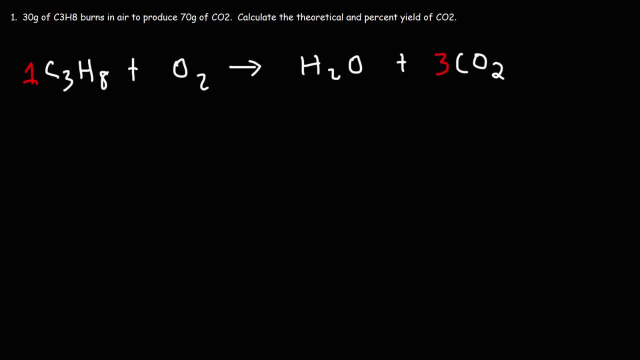 right Now. if we take eight and divide it by two, we're going to get four, which means that we need to put a four in front of H2O. So we get a total of eight hydrogen atoms on both sides of the equation. Now the last thing that we need to balance is the number of oxygen atoms on both sides. 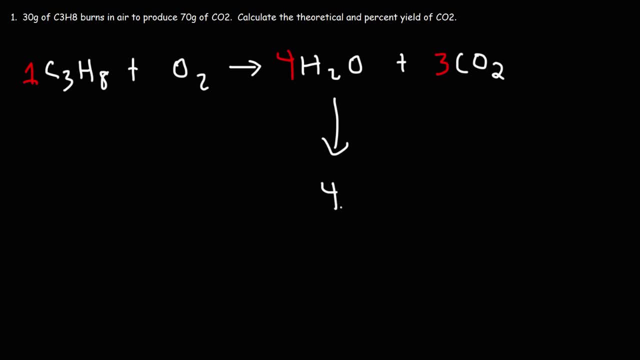 So in the four water molecules we have four oxygen atoms. There is an invisible one here, So you multiply the coefficient by the subscript and it gives you four. In the three CO2 molecules we have a total of six oxygen atoms, because if you multiply three by two you get six. So we 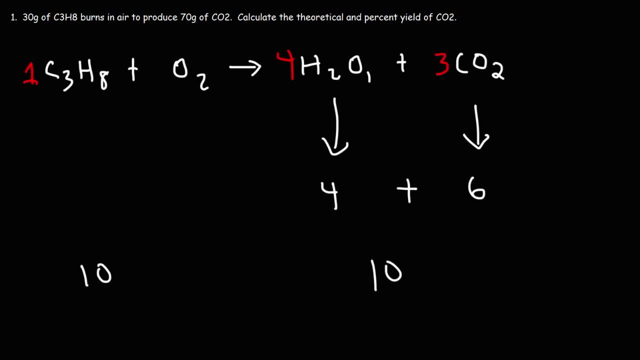 have a total of ten oxygen atoms, So we need ten on the left side. Ten divided by two is five, So we need to put a five in front of O2.. This will give us ten oxygen atoms on both sides. So now we 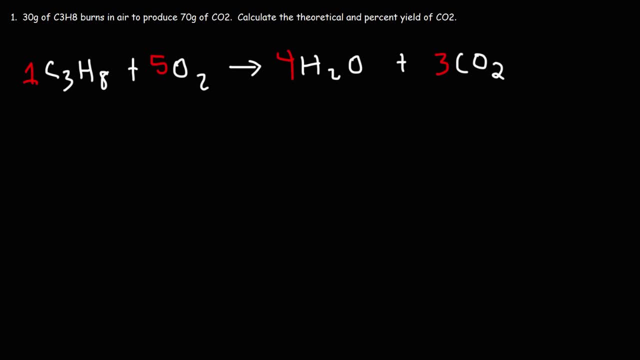 have a balanced combustion reaction. So now we can move on to the next step, and that is calculating the percent yield. So let's talk about the formula for the percent yield. The percent yield is equal to the actual yield divided by the theoretical yield times 100%. So that's the formula that we're going to use Now. 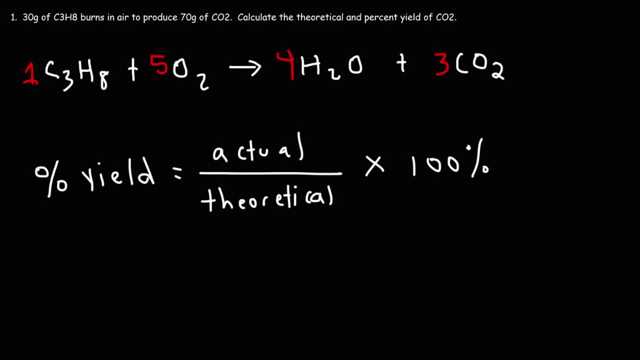 the yield typically corresponds to the product of the chemical reaction, And we have two products: water and CO2.. But in this example we're focused on CO2.. Now what is the difference between the actual yield and the theoretical yield? The actual yield is the amount of product that we actually got in the experiment. The theoretical 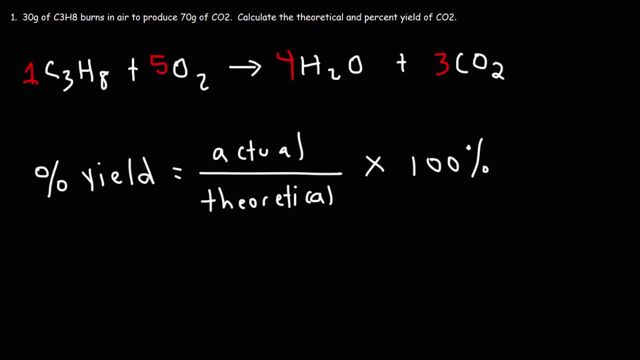 yield is the maximum that we could get if the experiment was 100% perfect, So keep that in mind. The actual yield is how much we get by experiment. The theoretical yield is the maximum that we can potentially get. Now. it's important to understand this, because the actual yield is not something that 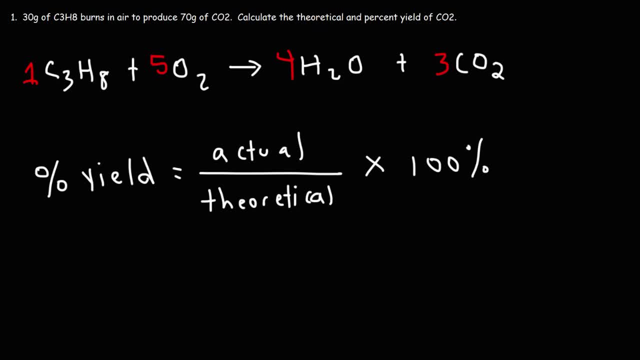 you can calculate without knowing the percent yield. In this problem we need to measure the actual yield, And so it has to be given to us in this problem, And it is In this reaction- we measure 70 grams of CO2 being. 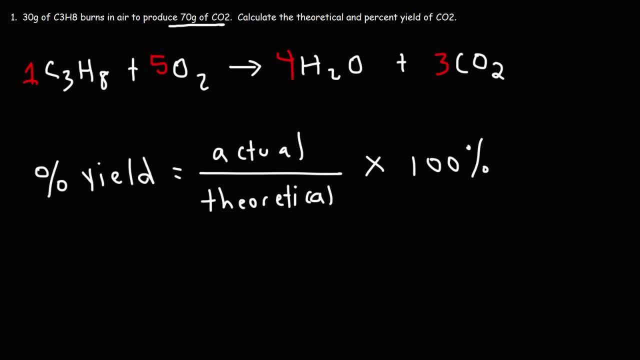 produced. So that is the actual yield. It's the amount of product that's actually produced in this reaction. It could be in grams or it could be in moles. What we need to do is calculate the theoretical yield, the maximum amount of CO2 that we can get in this. 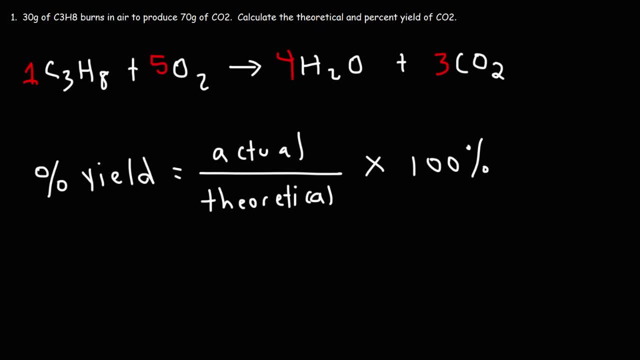 experiment. Once we have that, then we can calculate the percent yield. In order to calculate the theoretical yield, we need to convert the grams of reactant to the grams of product, in this case the grams of CO2.. Now, when working with these types of stoichiometric problems, you need to identify the limiting reactant and 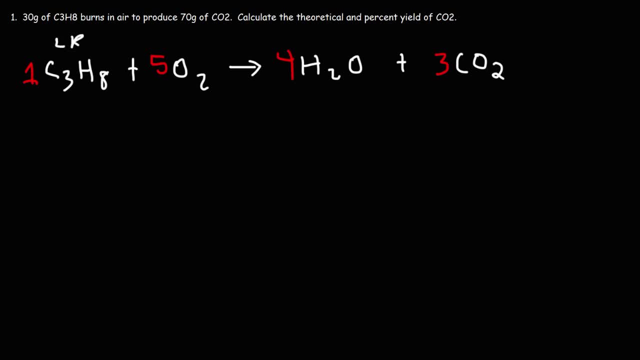 the excess reactant. The limiting reactant is propane. The excess reactant is O2.. Notice that we weren't given the grams of O2 that reacts with propane. It simply burns in air, And so we're assuming that there is a relatively unlimited supply of O2 in the 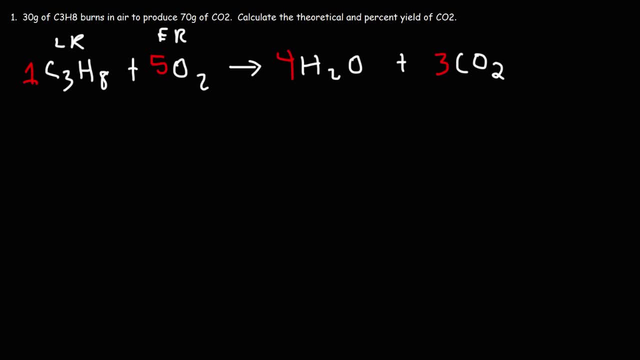 atmosphere. So O2 is going to be the excess reactant because we have so much of it in the air. So what we're going to do now is we're going to start with the information: we're given: 30 grams of the reactant propane. What we're going to do next is convert this to moles In order to convert grams to 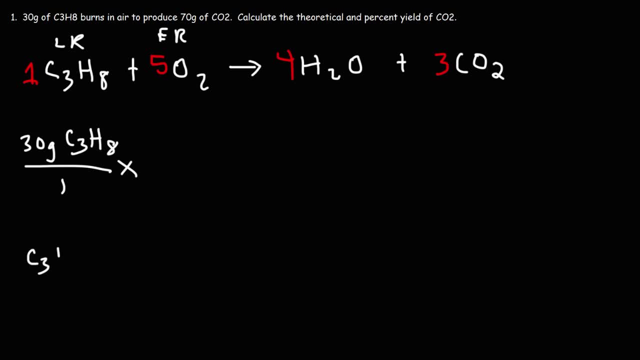 moles. you need to use the molar mass, So we need to consult the periodic table. Propane consists of three carbon atoms and eight hydrogen atoms. The atomic weight of carbon is 12.01, and for hydrogen it's 1.008.. 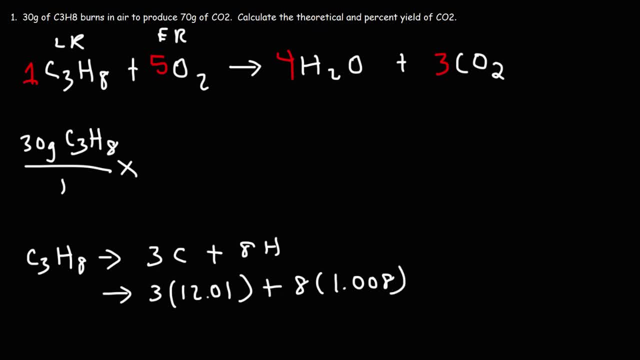 So let's go ahead and plug these numbers in. And so the molar mass of C3H8 is 44.094 grams per mole. So this means that 44.094 grams of propane is equivalent to one mole per mole. So one mole has a mass of that many grams. Now we need to set it up in such a 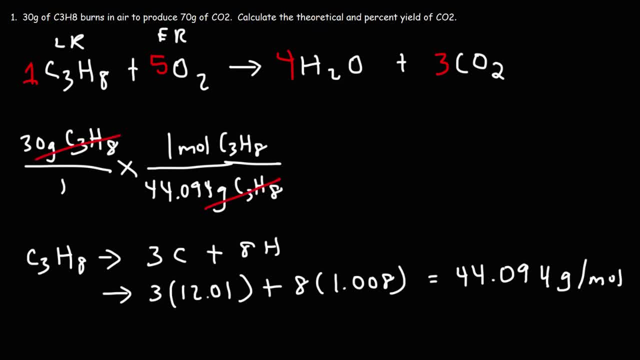 way that the unit grams of propane cancels. Now let's get rid of this and let's move on to our next step. In our next step, we'll need to change the substance from propane to carbon dioxide In order to go from one substance to. 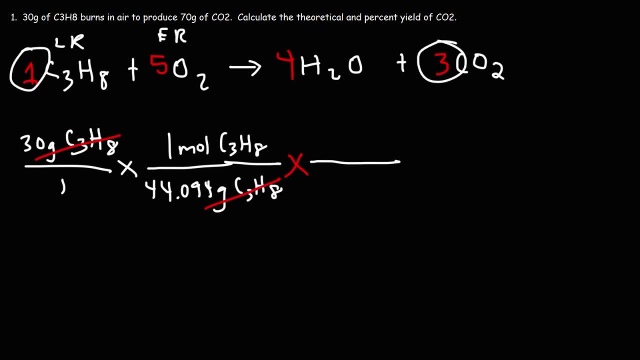 another. you need to use the moleration. So what this means is that one mole of propane will generate three moles of CO2.. So if we consume one mole of propane, in this reaction three moles of CO2 will be produced. 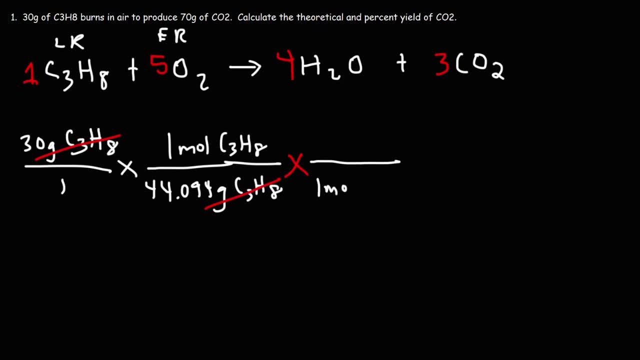 And that is the molar ratio between those two substances. Now we're going to put one mole of propane on the bottom, so that these units will cancel, And we're going to put three moles of CO2 because ultimately we want to get grams of CO2.. 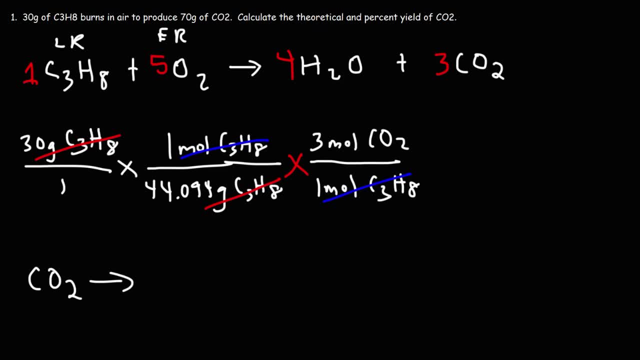 Now, in order to convert from moles of CO2 to grams, we need to get the molar mass, And so we have one carbon atom plus two oxygen atoms. We know that the atomic weight of carbon is 12%. The atomic weight of oxygen is 16.. 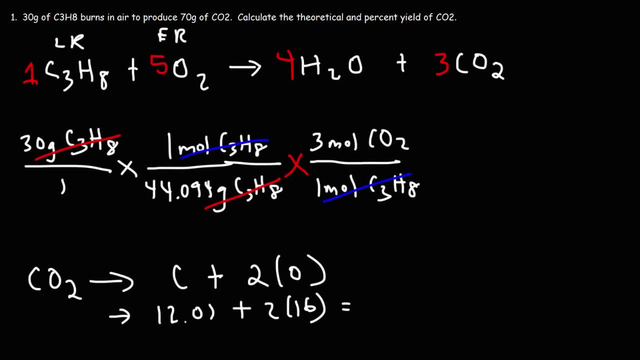 So it's 12.01 plus 32, which gives us a molar mass of 44.01 grams per mole. So this means that one mole of carbon dioxide has a mass of 44.01 grams, And now we can cross out the unit moles of CO2..